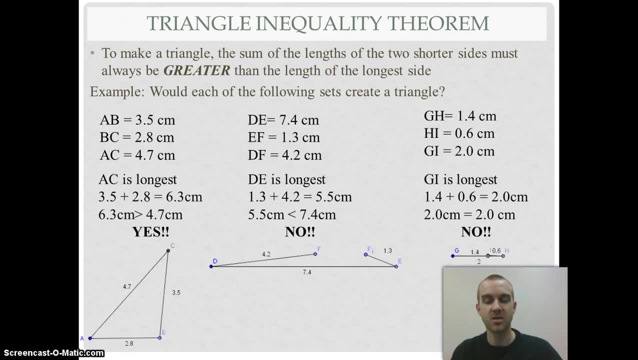 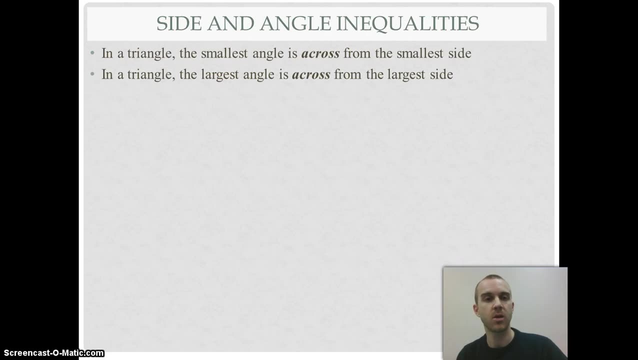 I have a segment Using segment addition postulate. So in essence what I'm saying is that GI plus IH will equal GH. That's segment addition postulate. So those two sides, when summed, have to be greater. Now another thing we know from the inequalities is that 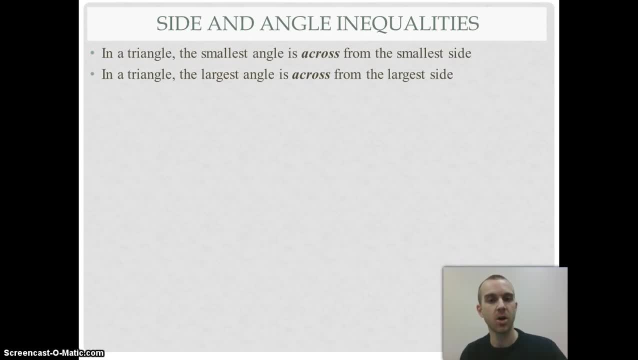 across from the smallest side is the smallest angle and across from the largest side is the largest angle, And that can be helpful. So if I want to take and order my angles from largest or smallest to largest, I look for My smallest side, which is the 2 and 65 hundredths. 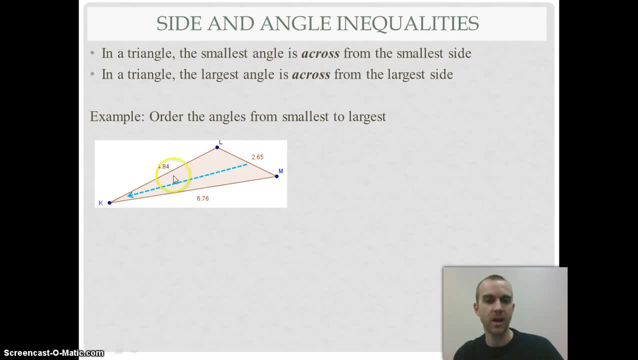 and opposite. it will be my smallest angle, angle K or LKM. Then my next one: I'm comparing: I've got 4 and 8, 8,400 versus 6 and 7,600.. So this 4 and 8,400. 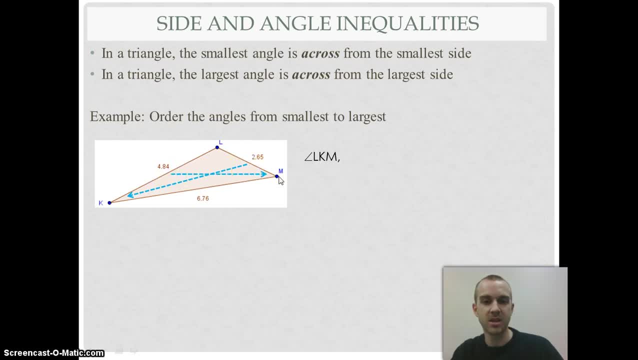 And I look opposite. So that'd be angle M or LMK, And that means my largest angle would be angle L, which I could also say is angle MLK. Now say, I want to order my sides from largest to smallest. So if I'm starting with my largest, I'm going to look for my largest angle. 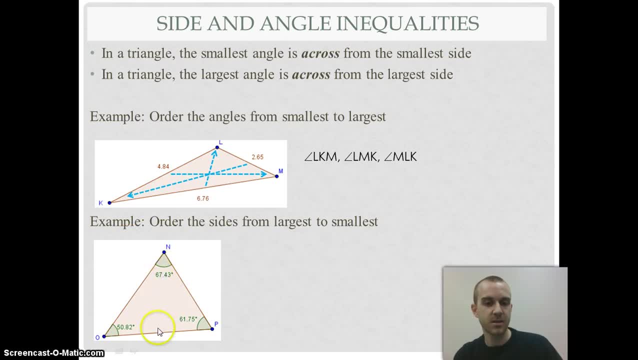 In this case that's angle N. So I'll look opposite it and I've got segment OP. Then I'm comparing angle P and angle O. Angle P is my next largest, so across from it is ON, which means my smallest side would have to be NP or PN. 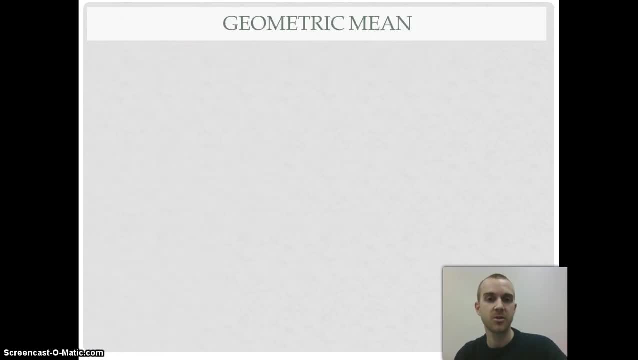 Now the geometric mean say I have three numbers that are part of a geometric sequence: an: A, B and C. What the geometric mean states is that if I create the ratios of A over B and B over C, so using that middle number twice. 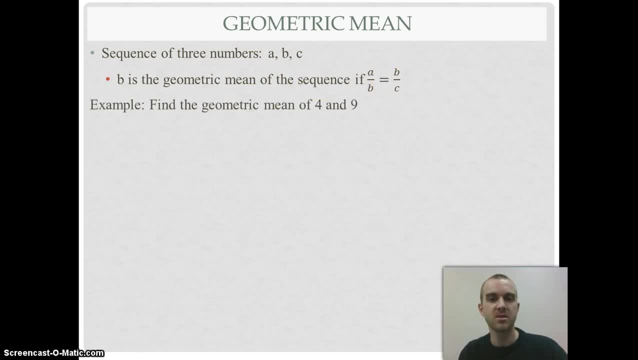 those two ratios need to be equal. So if I wanted to find the geometric mean of 4 and 9, so I would have 4, some value in between and then 9.. So I do 4 over X equals X over 9.. 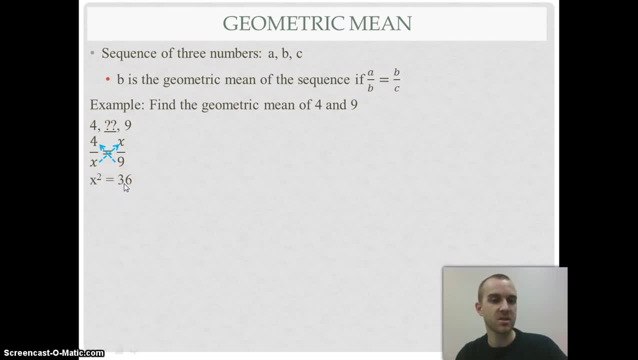 That gives me X squared equals 36, because I cross multiply, so X would have to be 6.. Now we can check that 4 over 6 is 2 thirds. 6 over 9 is 2 thirds. Both ratios equal 2 thirds. so I know that 4 over 6 equals 6.